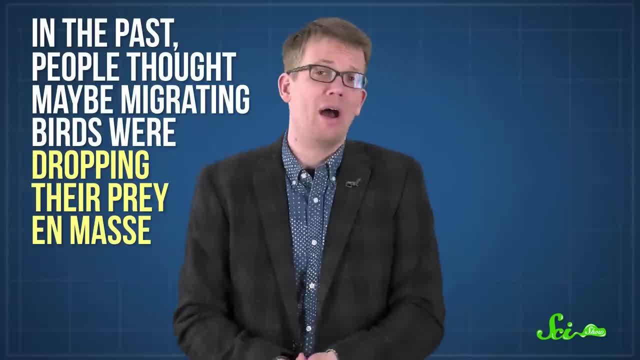 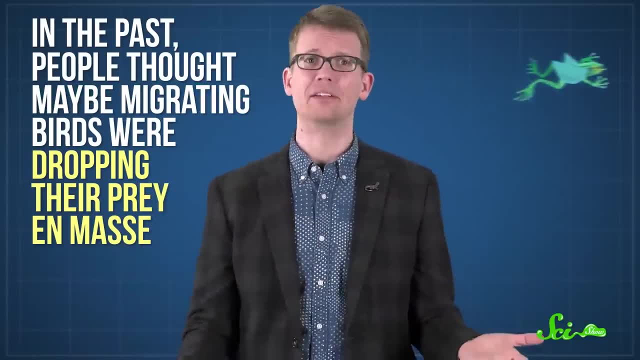 dropping their prey en masse. No one had any idea why they might do this, mind you, But why else would frogs fall from the sky? There's no such thing as a frog with wings. These days, most scientists and meteorologists think that these animals come from water spouts. 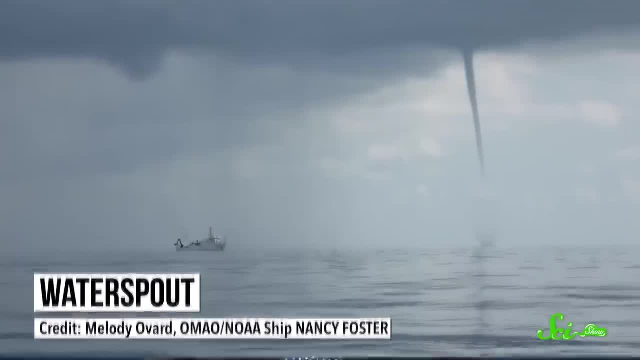 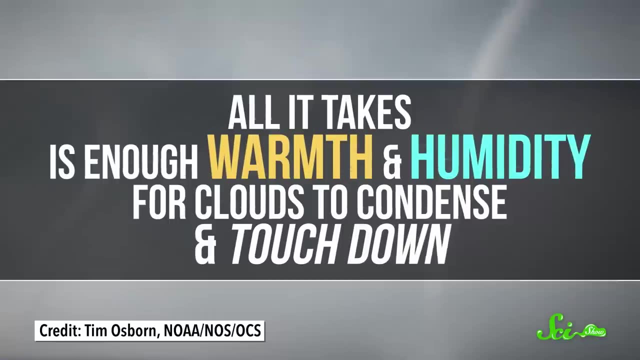 tornadoes over open water like oceans or large lakes. They're most common in tropical oceans, but they've been seen all over the world, and they can form over water even when conditions are relatively calm. All it takes is enough warmth and humidity for clouds to condense and touch down. 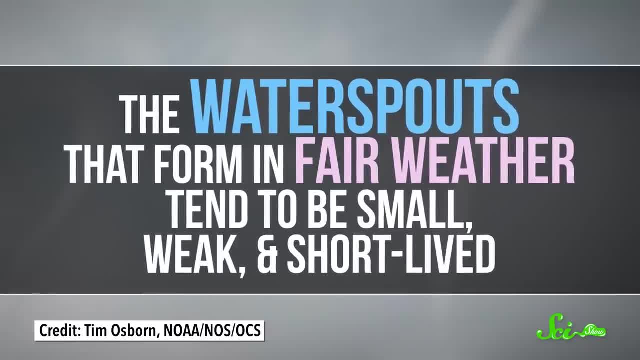 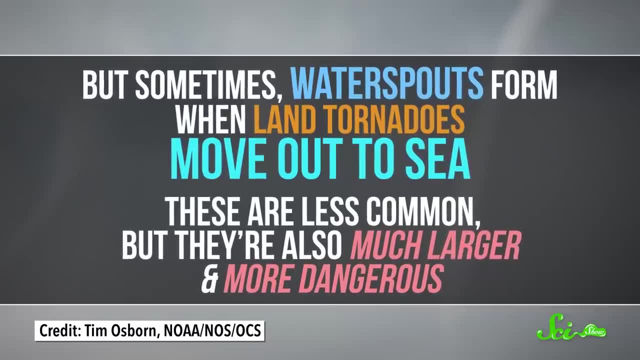 The water spouts that form in fair weather tend to be small, weak and short-lived, But sometimes water spouts form when land tornadoes move out to sea. These are less common, but they're also much larger and more dangerous. 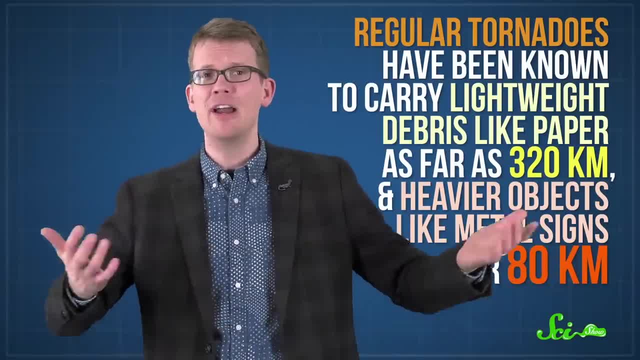 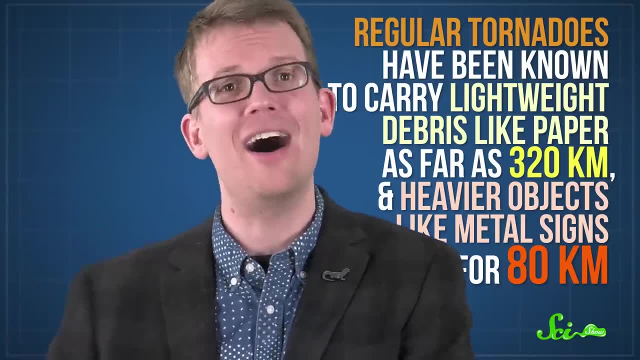 Regular tornadoes have been known to carry lightweight debris like paper as far as 320 kilometers and heavier objects like metal signs for 80 kilometers. I mean, Dorothy made it all the way to Oz. So while water spouts aren't usually as strong, 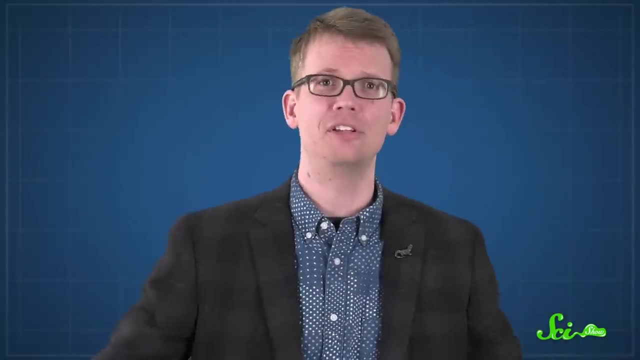 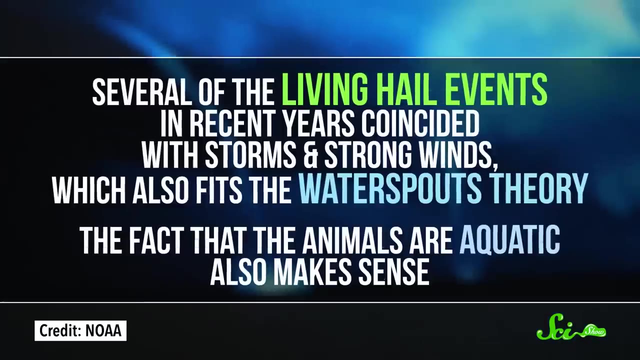 the idea that they might suck up things and transport them some distance and then drop them in a new location does make sense, And if they do, those things could include small fish or frogs. Several of the living hail events in recent years coincided with storms and strong winds. 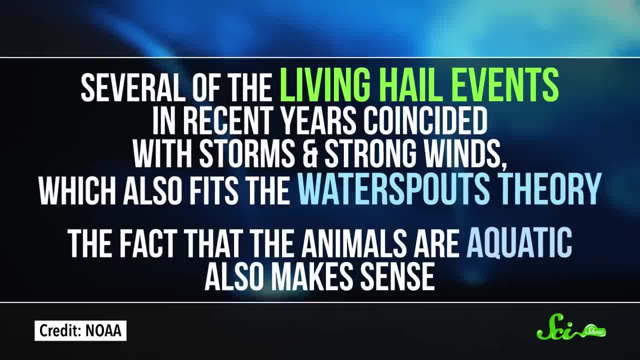 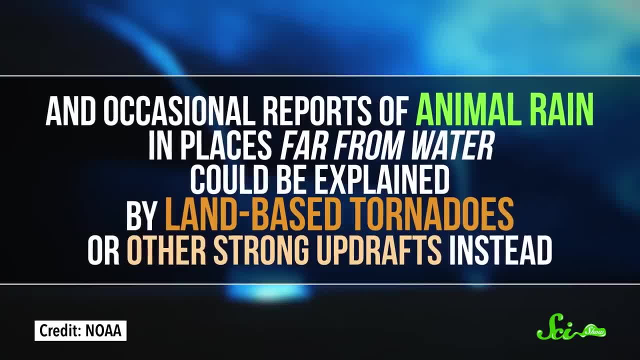 which also fits the water spouts theory. The fact that the animals are aquatic also makes sense, And occasional reports of animal rain in places far from water could be explained by land-based tornadoes or other strong updrafts instead. The thing is, no one has actually ever seen this happen. 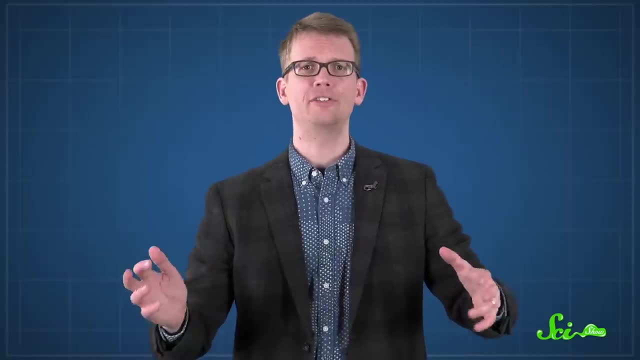 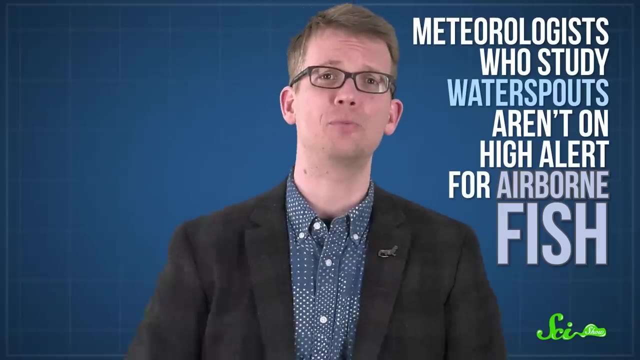 It isn't exactly easy to explain. We can't observe a violent storm over water, so it could just be that meteorologists who study water spouts aren't on high alert for airborne fish, Or since these amphibious rain events are just so rare, 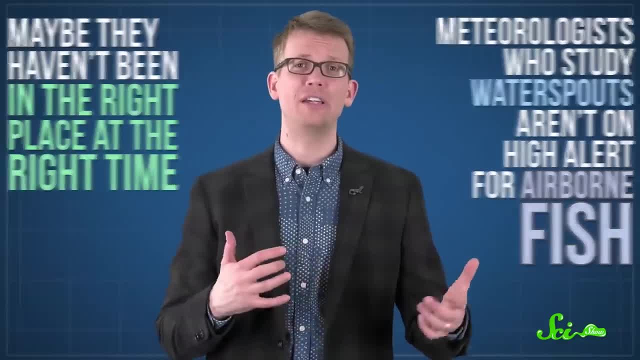 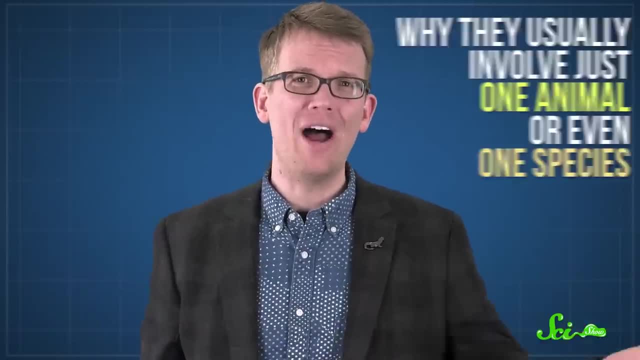 maybe they haven't been in the right place at the right time. So, even though the water spouts idea fits really well, we haven't been able to confirm it. Maybe if we did, we could also explain another mysterious detail: why they usually involve just one animal or even one species. 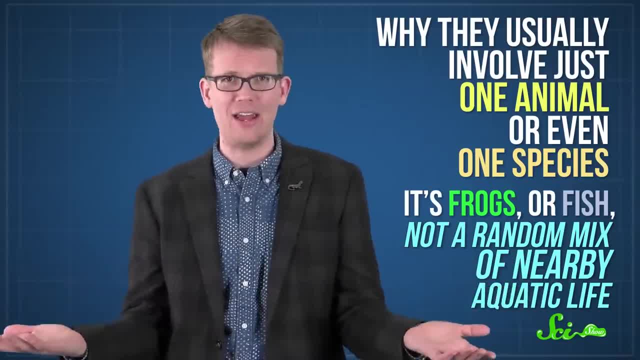 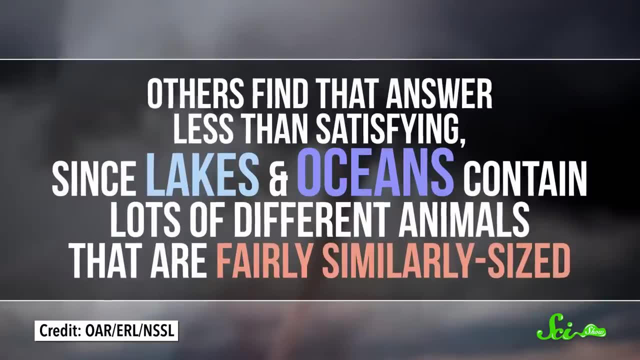 It's frogs or fish, not a random mix of nearby aquatic life. Some scientists think that that's because objects of similar size and weight fall out together as storm forces die down. Others find that answer less than satisfying, since lakes and oceans contain lots of different animals that are fairly similarly sized. 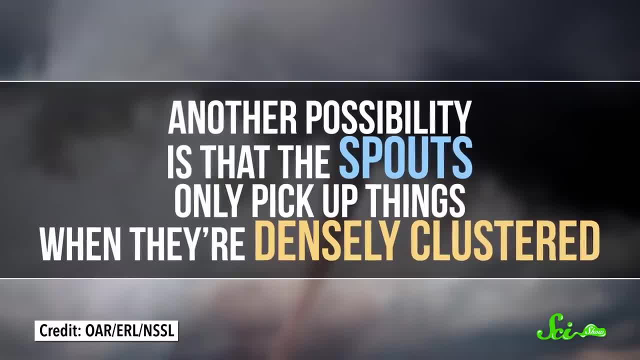 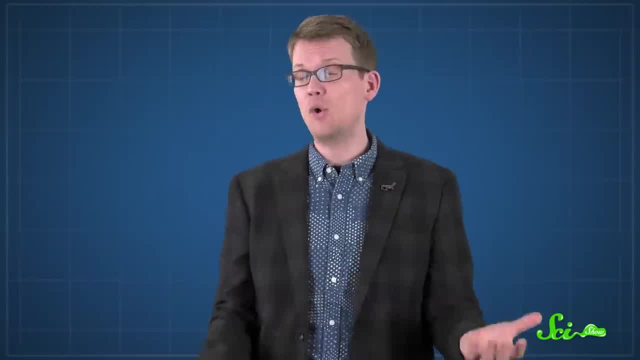 Another possibility is that the spouts only pick up things when they're densely clustered. But until we actually see animals getting pulled out of the water by spouts, no one can really say what limits the storm's catch. So if fish or frogs start falling from the sky, 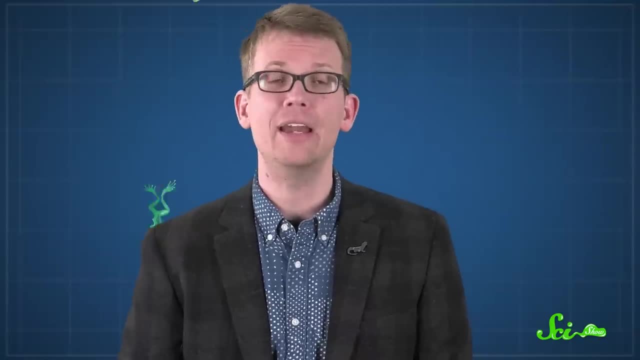 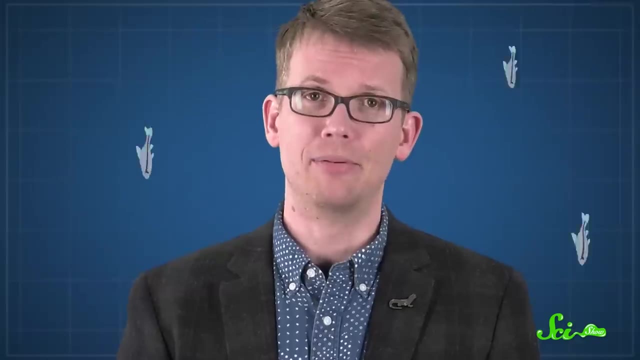 and plopping onto the sidewalk. don't panic, It's probably not a sign of the end times. It's just a really weird weather phenomenon with a perfectly reasonable scientific explanation, Probably. But even if it's not raining frogs, the science of weather is fascinating. 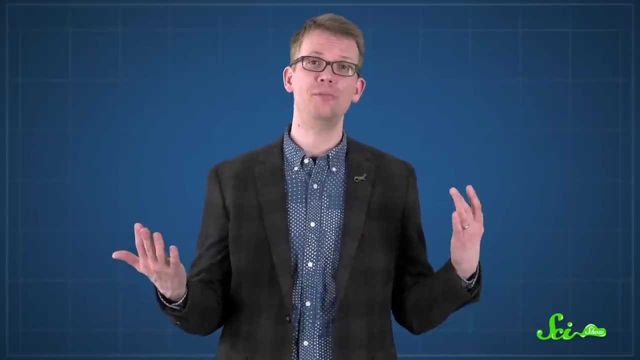 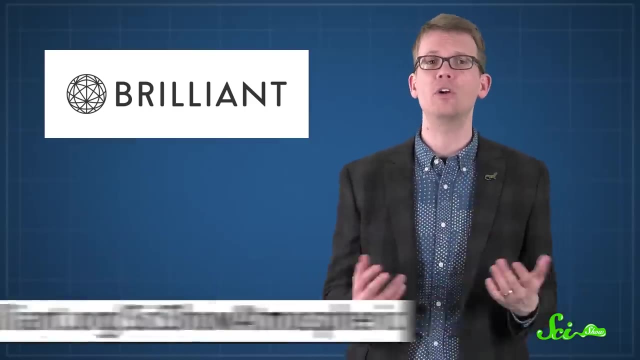 which is why I wanted to test my understanding of atmospheric pressure systems with this brilliant quiz. If you want to join me, Brilliant, set up a link so you can test your knowledge too. Click on the link in the description or go to brilliantorg. slash scishowatmospheric in a new tab. 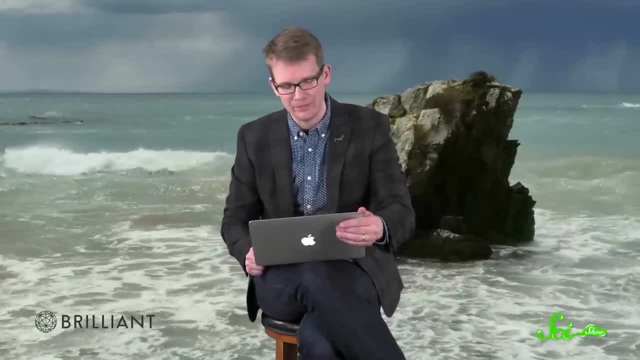 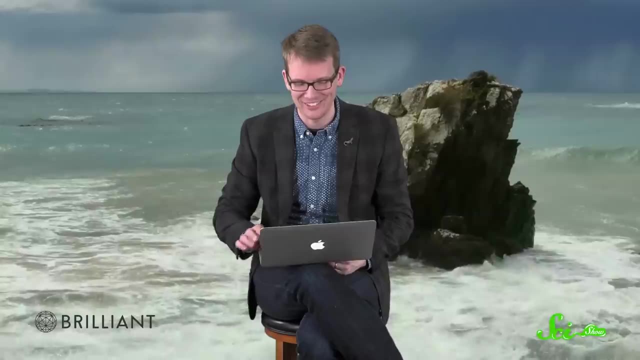 I'm taking the quiz. So I first got excited about meteorology when I was in college because there was a cute girl who was really into meteorology. This is how my interest in. It wasn't the weather that did it. So I'm taking my quiz here. 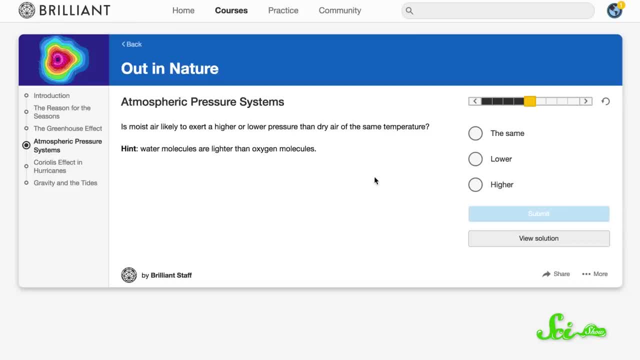 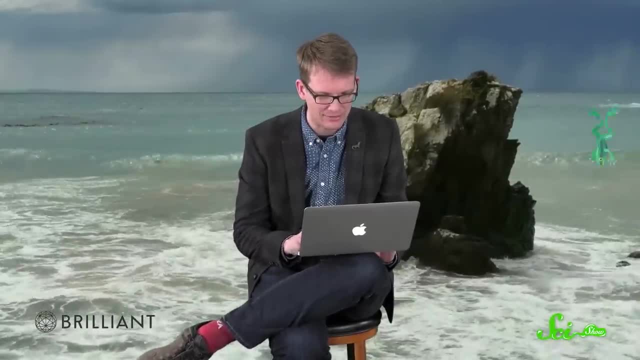 Is moist air more likely to exert a higher or lower pressure than dry air of the same temperature? Oh, hmm, I would say higher would be my guess, but now I'm guessing I was wrong. Moist air is lighter than dry air. 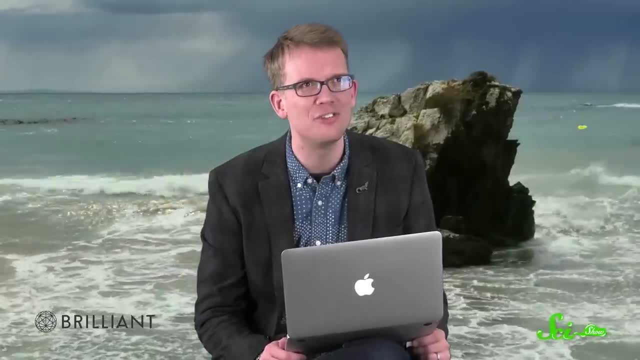 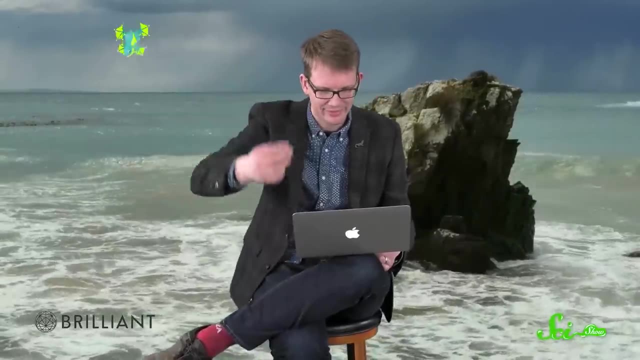 Huh, I guess because water is lighter than nitrogen, That makes sense. once it doesn't seem like that would be the case, I hadn't thought about that, which is why, like clouds rise up. Duh, Get your act together, Hank. 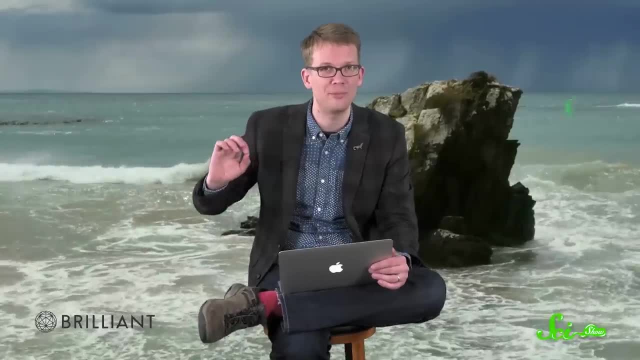 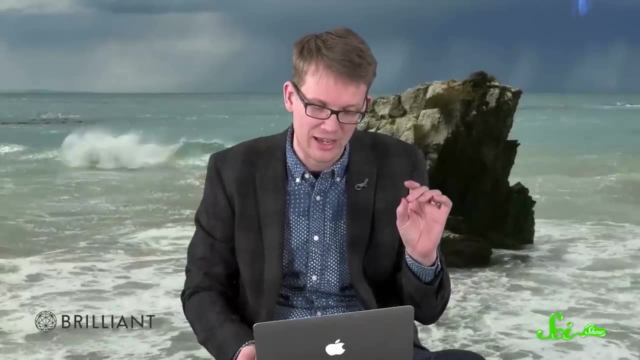 One of my favorite Twitter accounts is the National Oceanic Atmospheric Administration: Satellites Twitter. Very good satellite data coming out these days. I love it, but I feel a little bit like I don't actually know what's happening, even though this is my job. 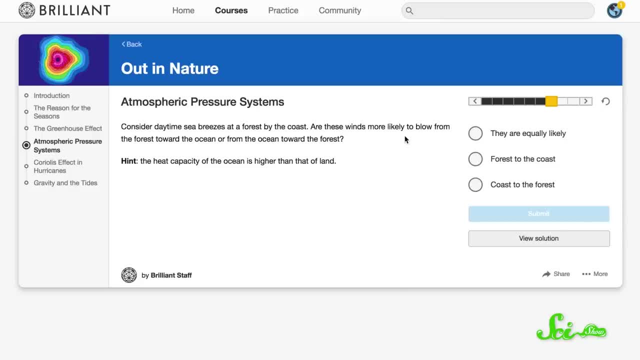 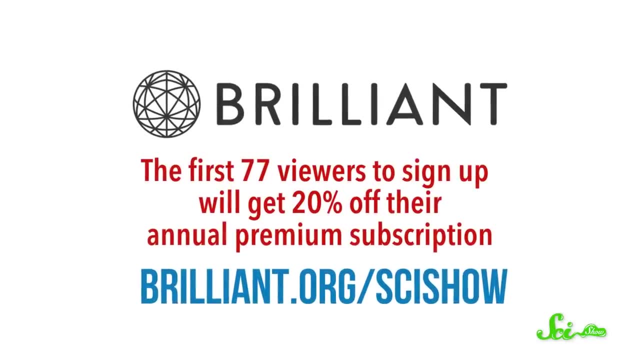 And I'm going through this and realizing that I indeed need to hone my skills To be a person who better understands what's actually going on. And you can do that too at Brilliantorg. The first 77 viewers to sign up at Brilliantorg slash SciShow. 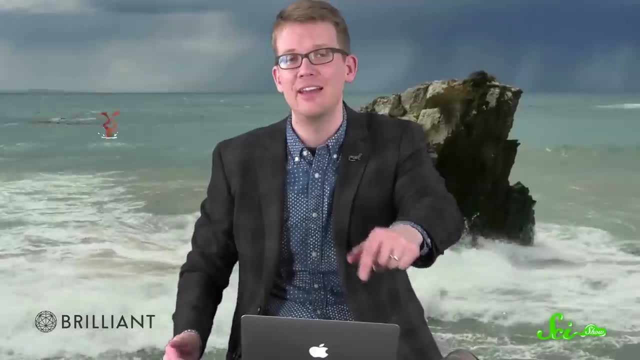 will get 20% off their annual premium subscription And you will support SciShow, So thanks.